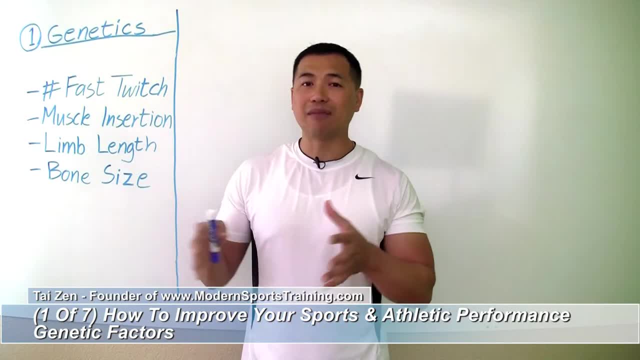 So let's go ahead and dive right in. I'm going to cover several different sections and this stuff is going to be very revolutionary, guys, because I'm mixing the Eastern and the Western methods of increasing the overall human performance here. okay, So let's go ahead and dive right in. 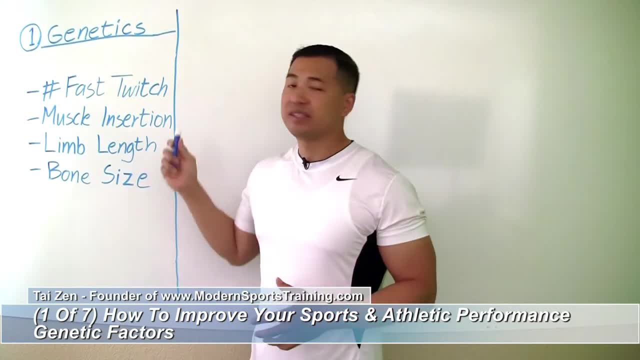 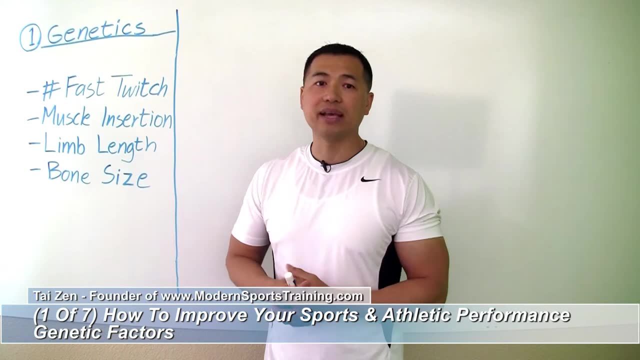 So the first thing I'm going to cover is the genetics. okay, There are several key genetic factors that makes an athlete stronger, faster, jump higher, do all these things okay, Without any kind of training whatsoever, just naturally they're born with it. 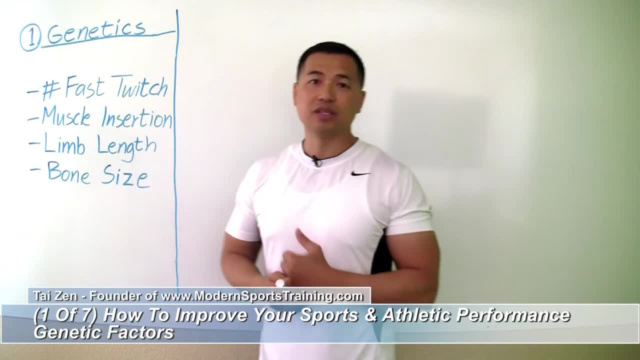 The first thing is the number of fast twitch fibers. If you're not clear on what fast twitch fibers are, just a quick review. The fast twitch fibers are the fibers in the human body that allows you to be explosive, to be fast, to be big, to be strong. 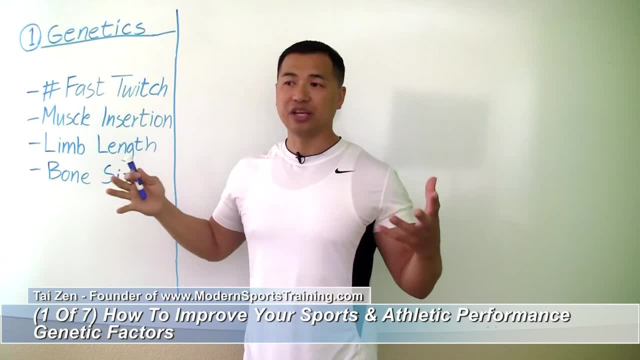 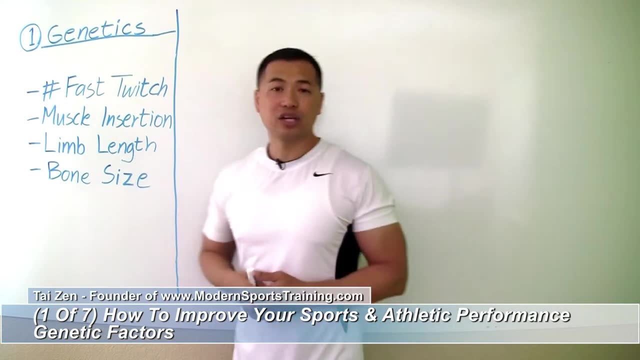 These are the fibers that grow inside your body to allow you to increase your sports performance. The other half of your body is created by slow twitch fibers and those fibers are not really that critical for you to train to increase your sports performance, unless you're looking for some endurance and conditioning. 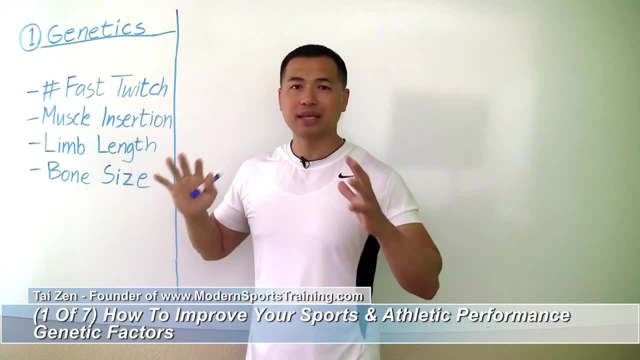 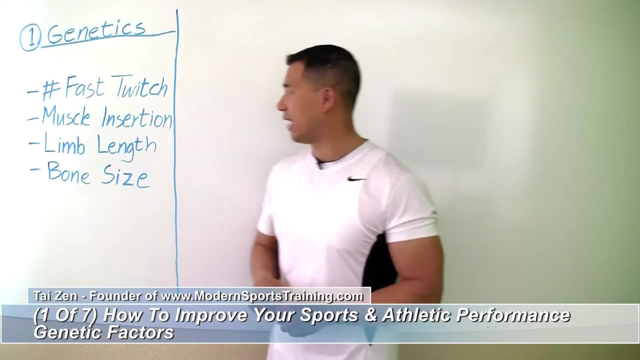 This is where the fibers that make the biggest impact in your sports performance. right here, All the professional athletes have a very high number of fast twitch fibers in their body That is a little bit above the average of what normal human beings like myself and others have. okay, That's what makes them a professional athlete. 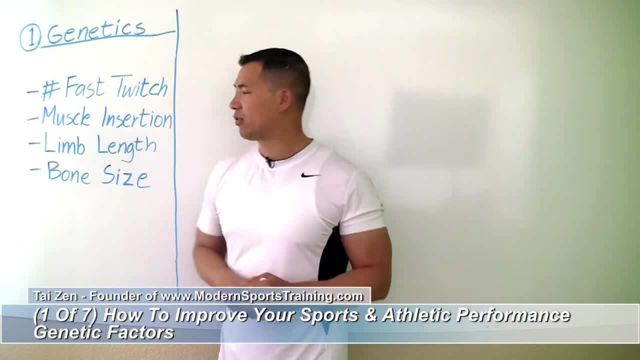 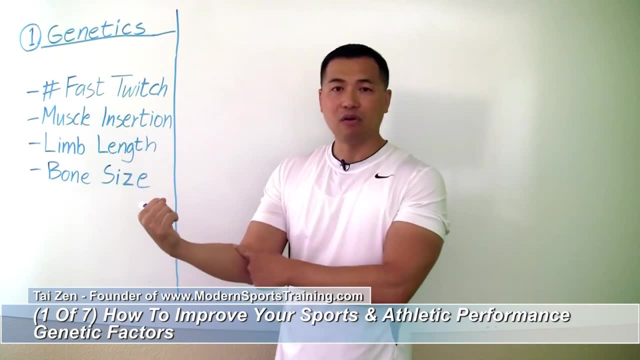 Now, one of the things. the other thing too- is the muscle insertion. okay, For example, if you look at where my bicep is at, where the bicep tendon inserts into your forearm, makes a huge difference in your sports performance. 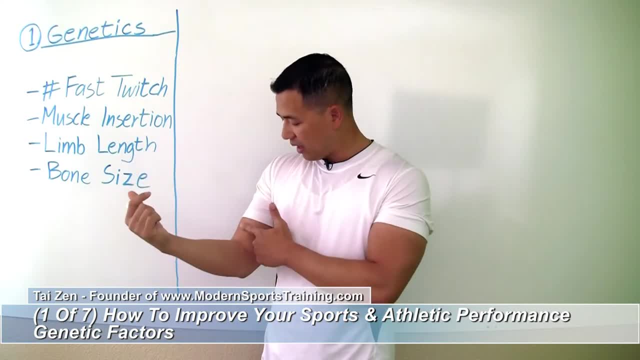 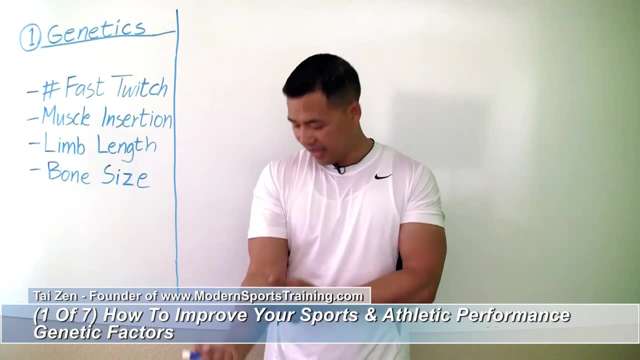 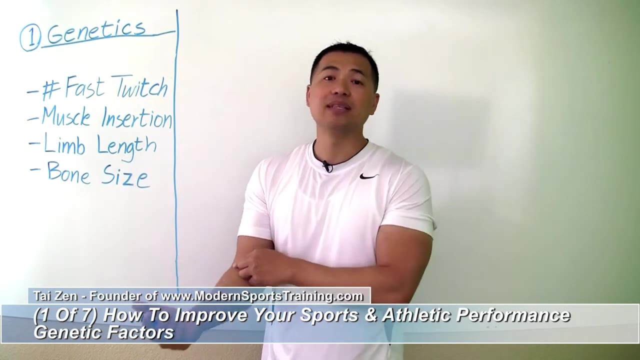 For example, if you want to be strong, then your bicep tendon will attach lower down here, Which allows it to have more leverage to pull more weight. Now, if it's attached higher up on your forearm, then what happens is it doesn't have that much leverage, but what it does is it has a lot of speed. 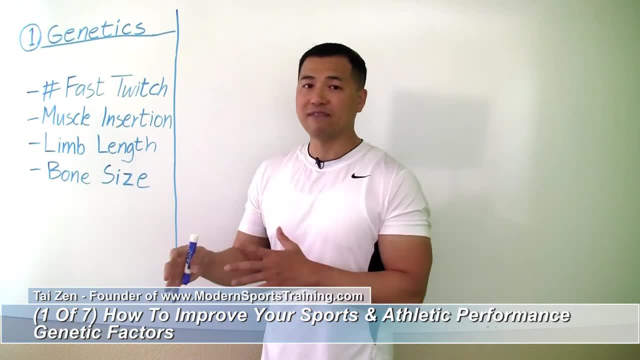 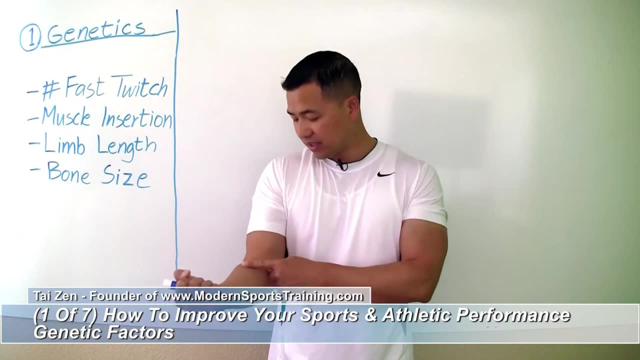 So someone like Bruce Lee or somebody like that that can move their hands very fast, or any of these professional fighters in the UFC, what happens is their bicep tendon is, most of the time, it's situated just slightly higher, And we're talking about just millimeters, guys. We're not talking about inches or anything like that. 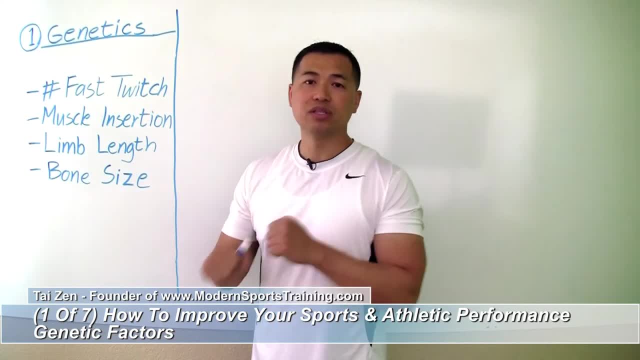 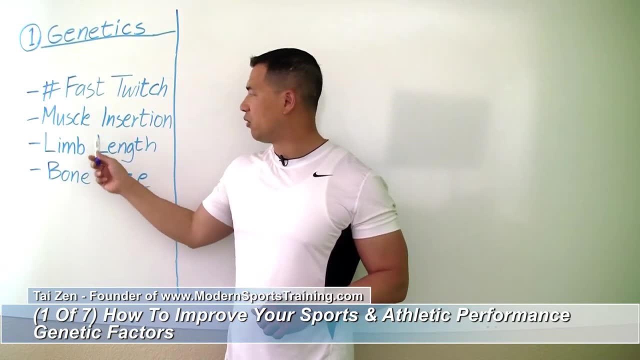 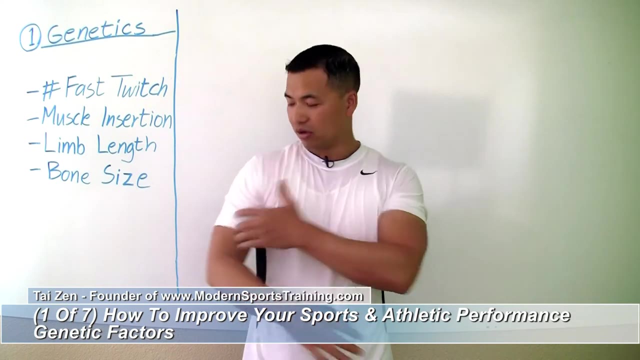 But it makes a huge impact on the leverage that they have In their bones and their limbs to be able to kick and punch faster or to be able to just move faster, alright. The other thing that is also important is your limb length, And what I mean by that is the length of your arms or the length of your shin bone or your thigh bone or your humerus bone or any of that. 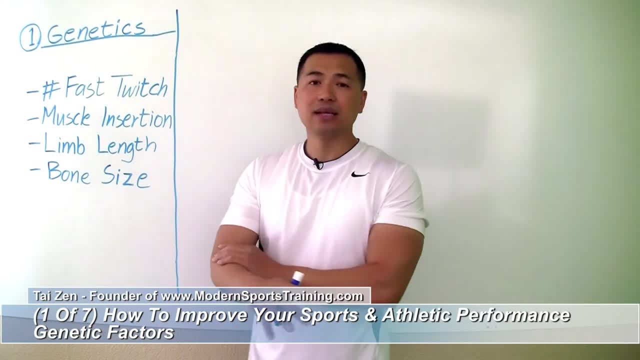 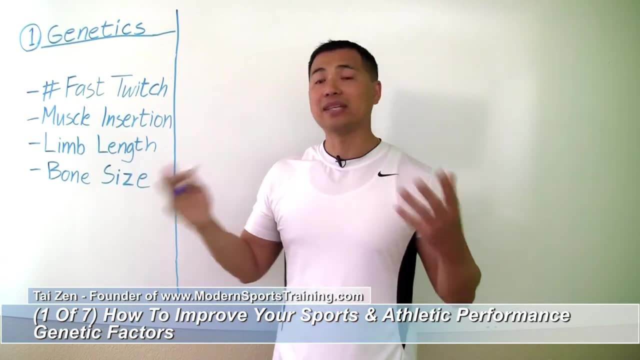 What it does is that the longer the length is, the more leverage that you have And, depending upon with the combination of where the muscle is inserted into that bone, it has a huge impact on how fast you can move that muscle. So that's one of the things that I want to talk about. 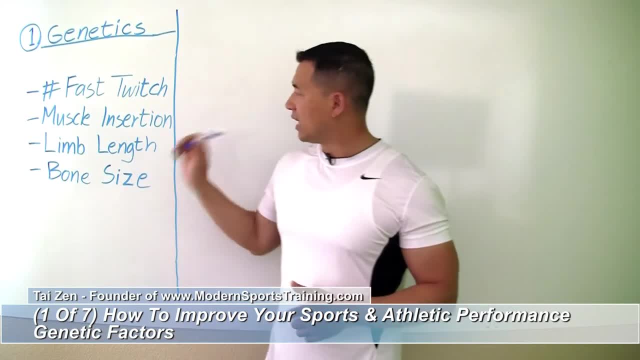 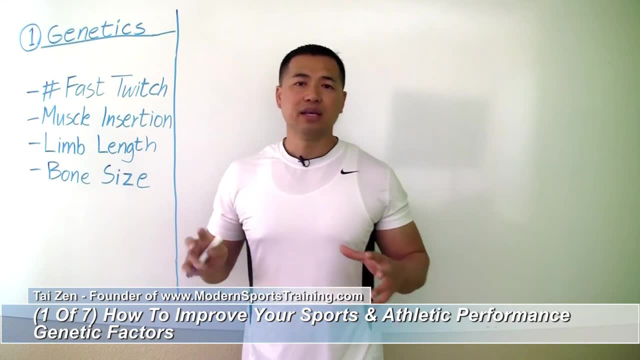 How fast you can move your hands or your legs, And the other condition factor that you want to look at- that's genetic- is your bone size. This is something that hardly anybody ever talks about. is the bone structure that you have to be a professional or a high-performing athlete? 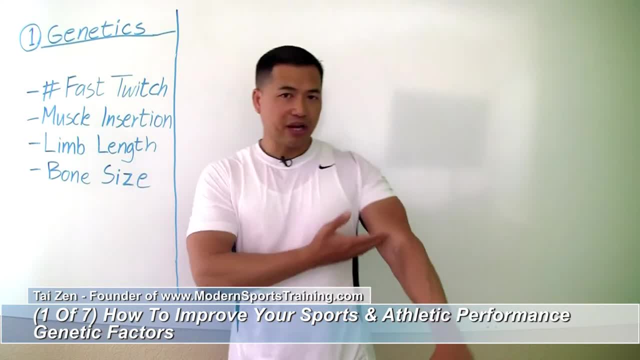 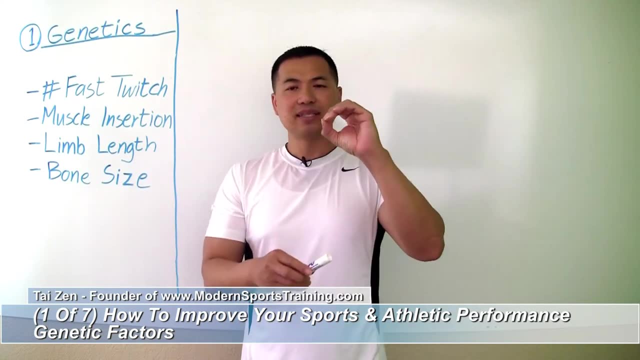 And what I mean by that is this: If you do a cross-section of my arm and let's say that you cut my arm in half and you look at the side view of it, you might see like a this big of an arm right in the- excuse me- right here. 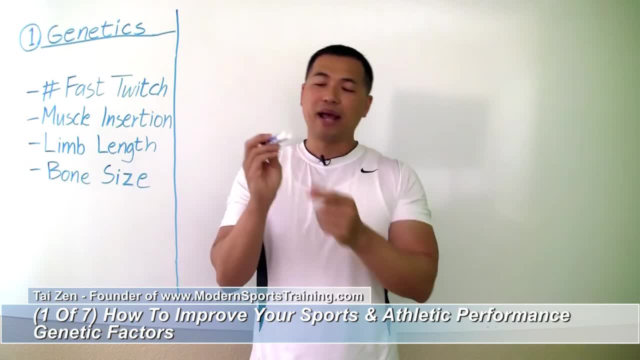 If you have a bone, that's this big right. what happens is you have this much bone and look at how much empty space there. Let that represent the muscle fibers. okay, Someone that has a small bone will have denser muscles. So right now I have like 16 and a half inch arms, okay. 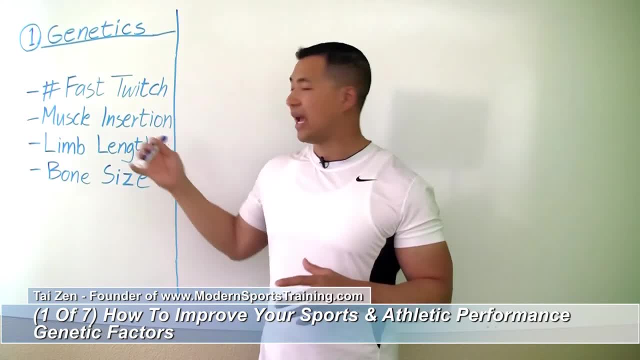 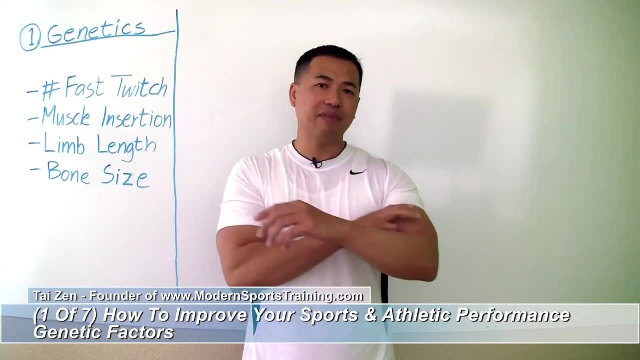 So if you take someone else that is genetically gifted to have more muscle, more strength and more power, what happens is the muscles they'll have the same size: 16 inch and a half arms like I do, except their bone is smaller. 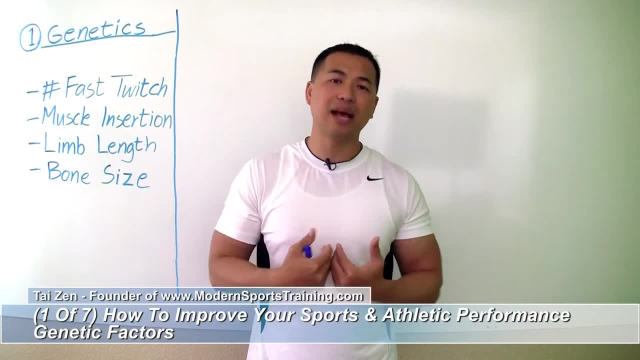 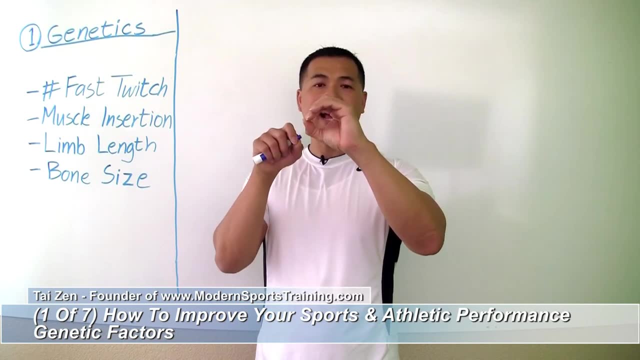 So if the bone is smaller, then they have more muscle in that arm than I would. So that's very important. And to give you a view, if this was my arm here and my bone is this big and then another guy has it and their bone is only that big inside the muscle, 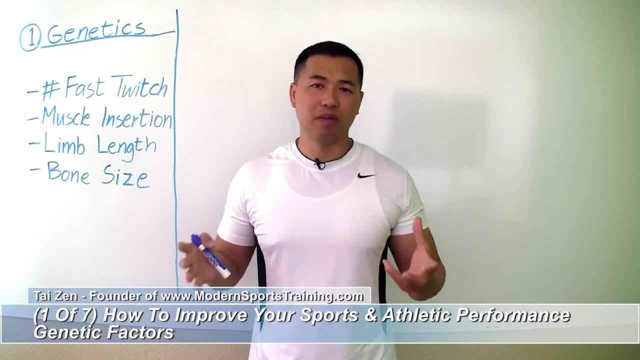 what happens is that allows you to have more muscle, And I don't know if you guys can see that in the video or not, but let me do it here in front of my shirt, so you can see it. So this is here. 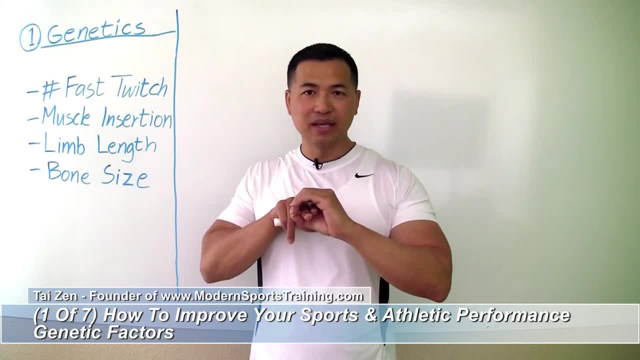 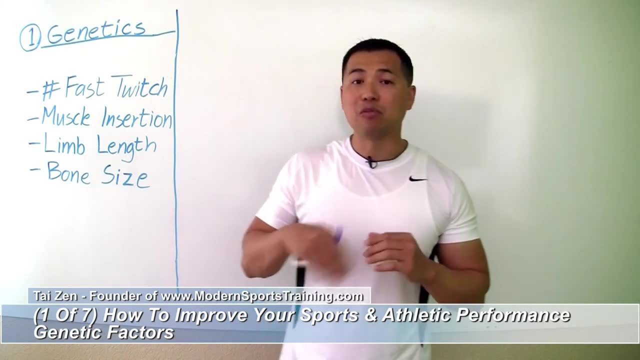 This is the muscle right here and the bone in my arm is this big. You notice that there's not too much room left for muscle. If someone else has a bone that big, there's a lot more room left for muscle around it, So they're able to produce more power, more speed and a bunch of other stuff and more strength, okay. 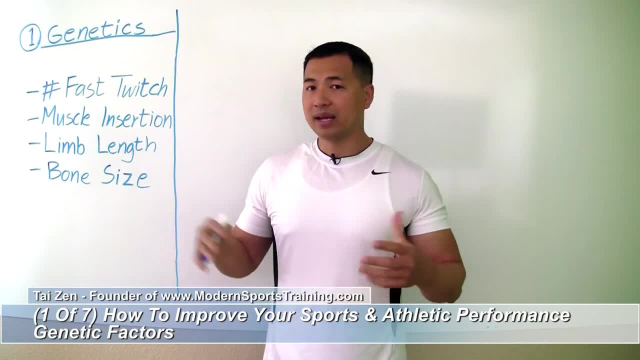 So these are the genetic factors that we talk about right there, And I don't want you to focus on this, because either you have it or you don't. There's no type of training that I know of or that I have seen or researched. 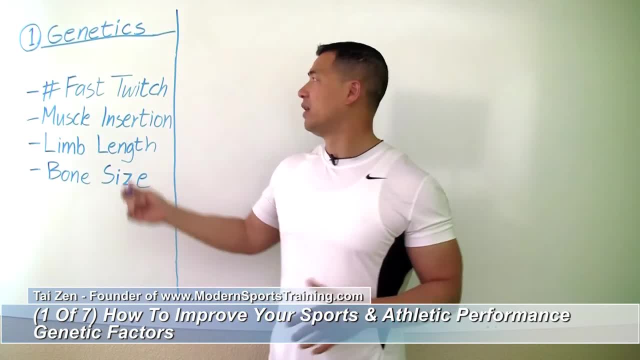 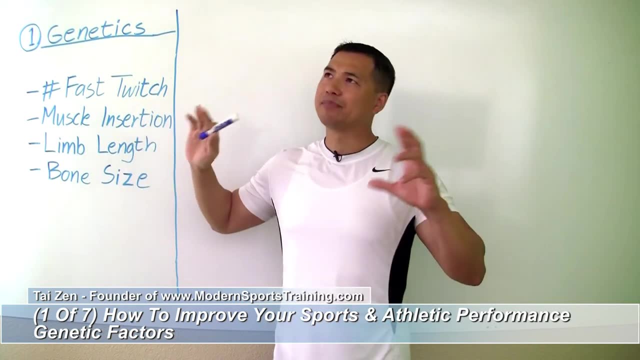 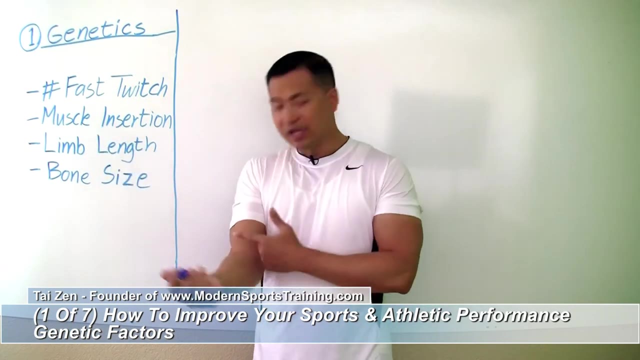 or actually witnessed myself or used myself that can increase the number of fast twitch fibers, the muscle insertion. This would have to be done with surgery. In the past I've done some research where some of the Russians and the Germans would operate and remove somebody's tendon and then reinsert it to a different area to test. 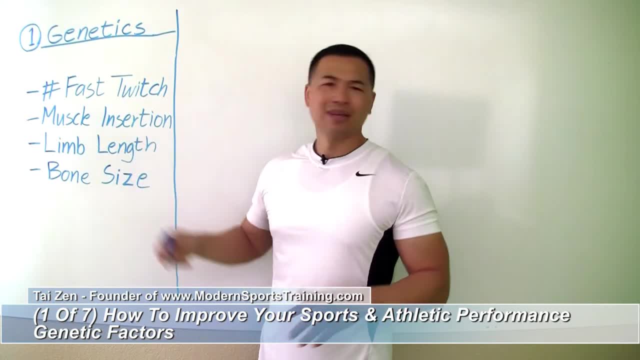 and see if they get more speed and more strength and stuff like that. I'm not even going to talk about that because that's not something that you can do at home or anywhere in America or in any country that I know Without costing a lot of money. okay, 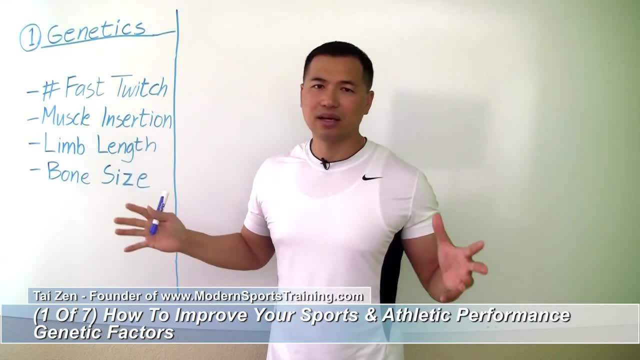 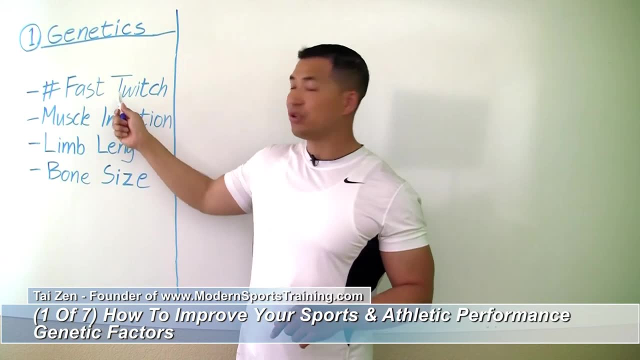 The other thing too, is your limb length, your bone size. none of that you can change alright. So that's it for genetics. These you cannot change. Now there's, oh, by the way, the number of fast twitch fibers that can be changed if you train early enough. 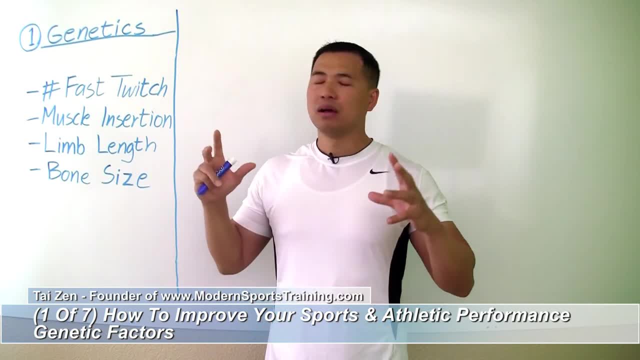 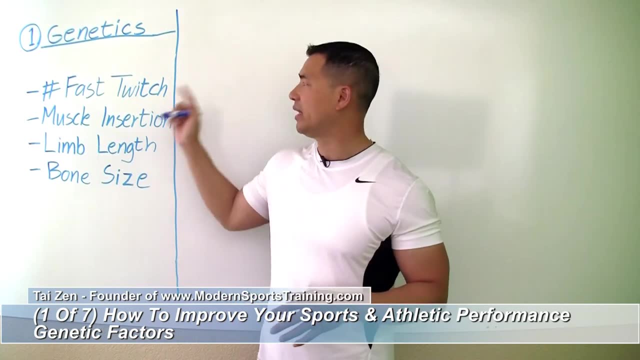 If you do some weight training, gymnastics, any kind of martial arts training, anything where your hands and your body has to be very explosive and it has to move very quickly, you can increase the number, The quantity of fast twitch fibers before you hit puberty. okay. 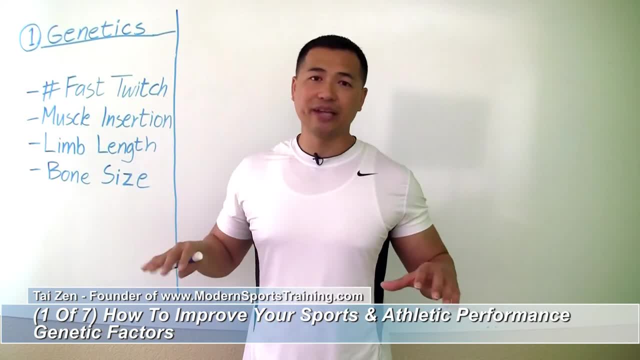 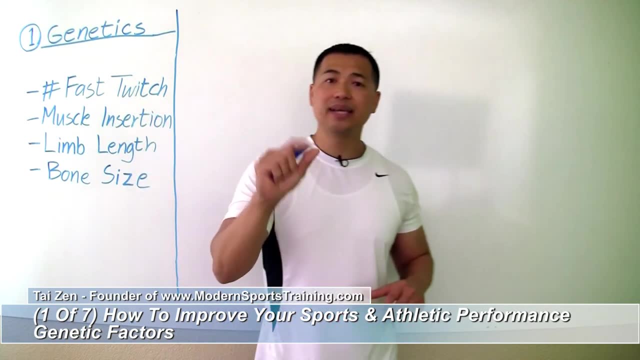 After you hit puberty and you're an adult, there ain't no changing it. You can increase the size. you can increase the size of it but not the quantity of it. So this you can do slightly before you hit puberty, okay. 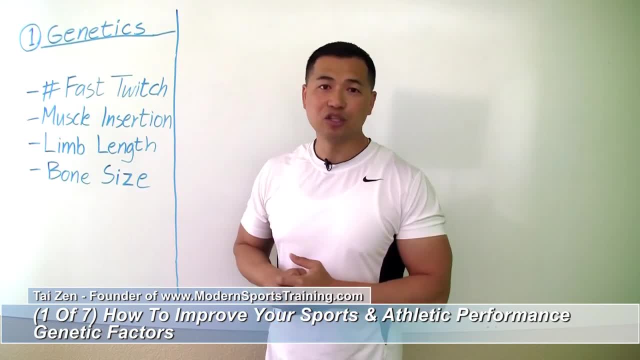 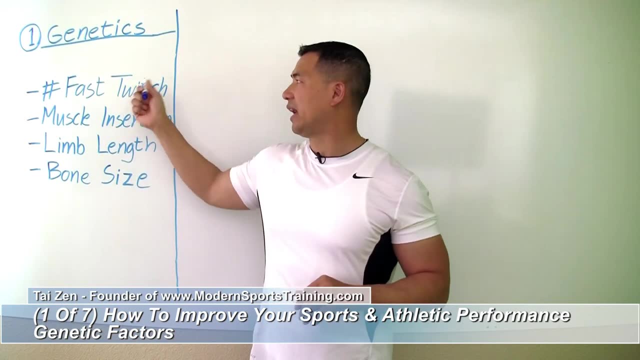 So if you're a teenager watching this, or you haven't finished puberty yet, or you're a parent, a coach, a trainer, anything like that, and you work with people that have not finished puberty, you have a means, a mechanism to influence how many you know. 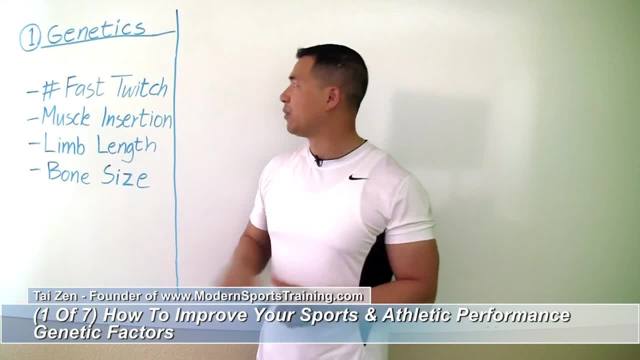 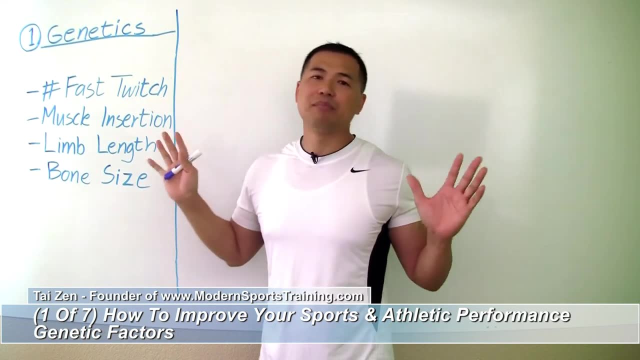 how many fast twitch fibers they have in their body. okay, But that's basically it. I just want to mention really quick about the genetics, because this is an area that there's not much you can do to change it. okay, Either you're born with it or you don't, okay,